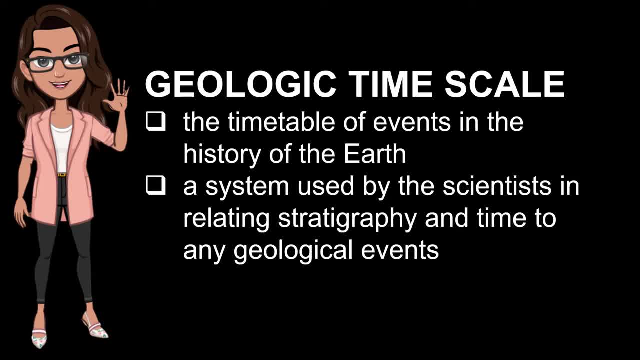 The geologic timescale is subdivide into geologic time units. i everyone break ingredients carpet: Eon, era, period, epoch. This units are based on stratigraphy, Which is the description of rock succession and its Interpretation in terms of a general timescale, which is the basis of historical geology. 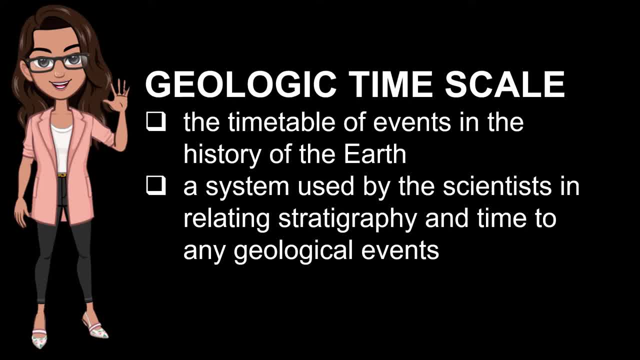 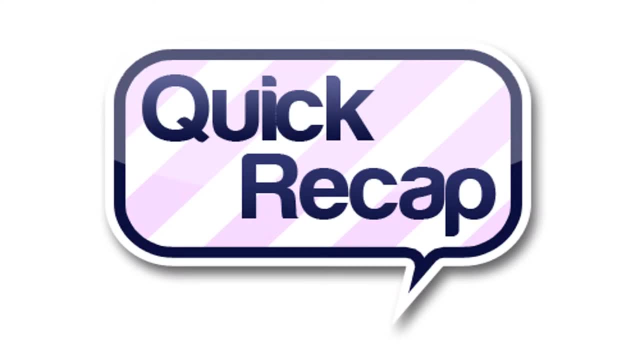 The use of indexes. fossils plays a very important role: the study of geologic time scale. they serve as indicators of specific geologic periods. as a quick recap, in the previous lesson you have learned that fossils are important in understanding geological changes through biostratigraphy correlation. 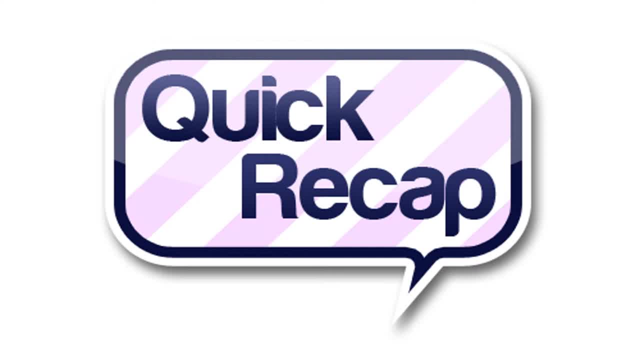 which help geologists match layers of rocks in different locations based on their similarities. you have learned two methods which geologists use in identifying the age of rocks. one is the absolute dating, wherein the exact age of rocks or fossils are determined through radiometric dating method. the other one is the relative dating, where fossils 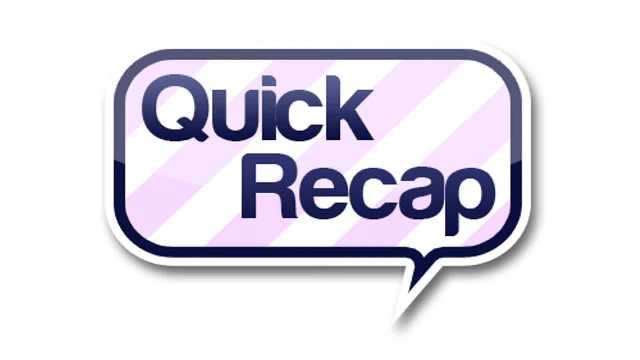 are compared to something for which its age is already known. these methods are very important in arranging geological events and the rocks that were left behind in a sequence. it is through these mechanisms that help geologists generate the geologic time scale. now you will continue learning more about geologic time scale as you go through this module. 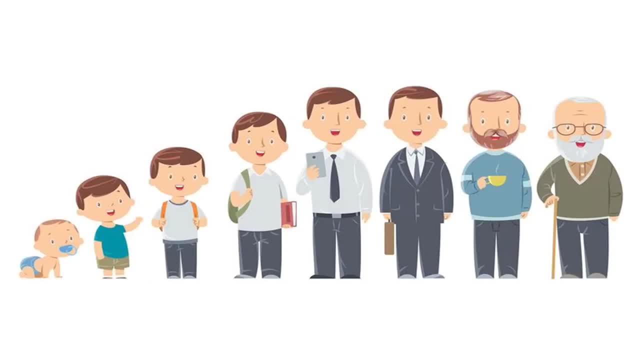 the study of human development includes different stages, starting from prenatal to old age. the development is important in understanding how we learn, mature and adopt. some aspects of our life may change very little over time, while other aspects may change intensely. we are making our own life history, as we recall and jott 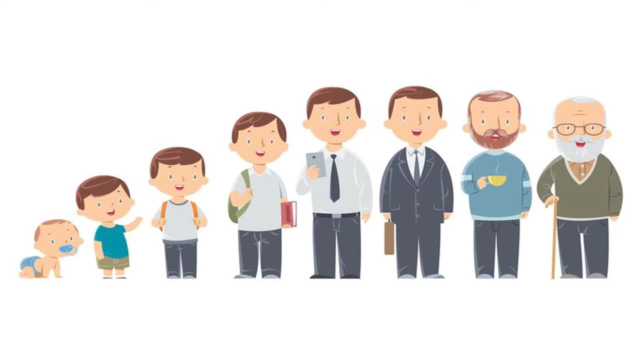 down the significant events that happen in our life. the history of the earth is compared to our life's history. events in our life, in every stage, expand as we get older. these events are, or characteristics are, a basis of how a person matures. also a basis for tracking the age of. 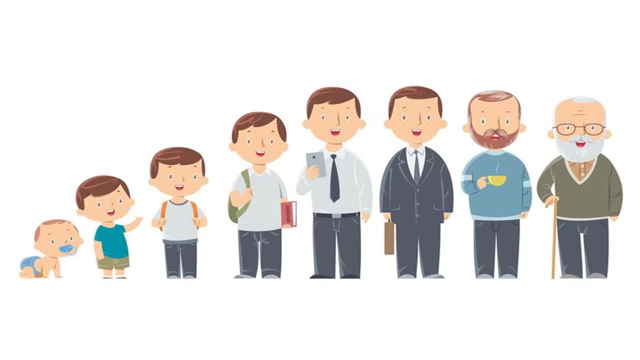 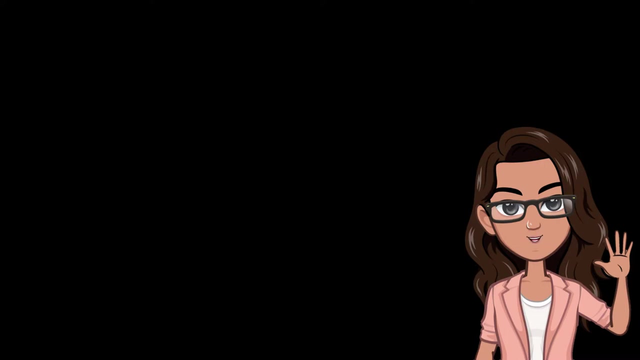 our maturity of an individual. in the history of the earth, fossils are Nuo rach layers and important events mark how long and how the geologic time scale was divided and lasted within a period of time. now you will learn more about this. the earth's history in reference to the geological time scale is divided. 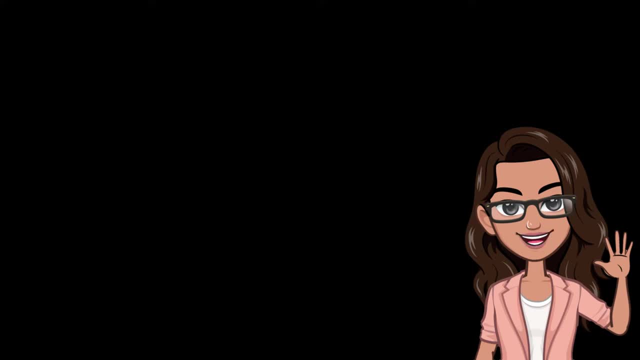 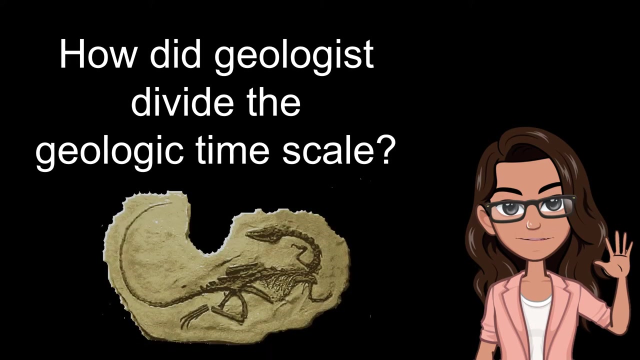 into different subdivisions with different time intervals that are not equal in length. geologists divide a geologic time scale. significant events in the history of the earth, fossils and rock layers were used to divide the geologic time scale. fossils, which are remains of ancient life, like plants and animals, as 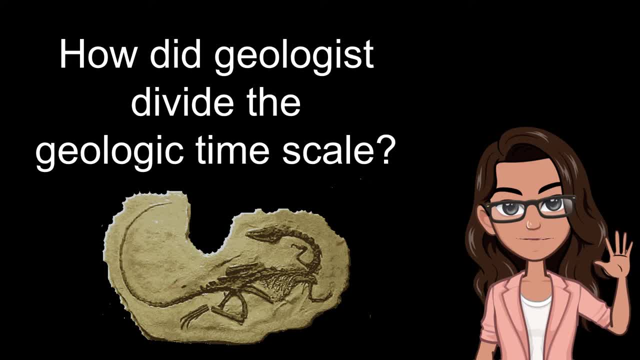 mentioned play a very important role in gathering important occurrences of facts and information about the existence of life and in the understanding of geological changes. index fossils that were preserved in rocks were used as indicators of certain geologic period. geologists usually relate the age of rocks with the age of fossils found in a certain area. isn't so great how the 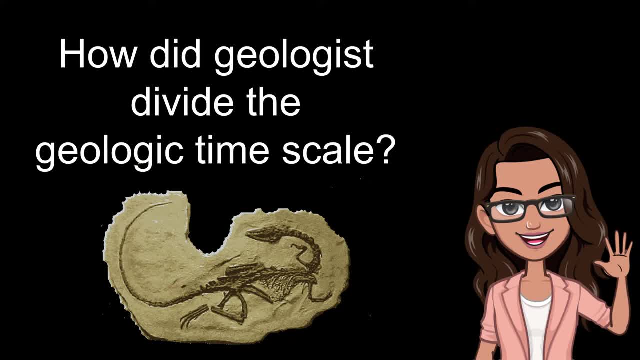 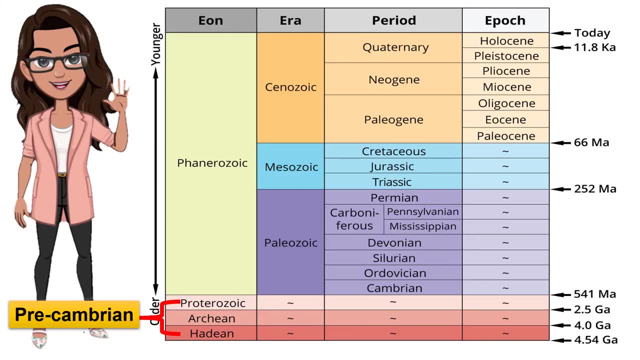 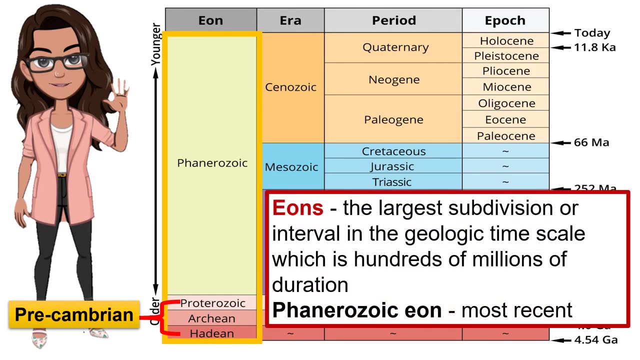 Earth's history was made. fossils and layers of rock are important in the determination of the ages. now let us continue learning. let's talk about the major subdivisions, for stop is a eons. eons are the largest subdivision or interval in the geologic time scale, which is hundreds of millions of duration. the panerozoic eon is the 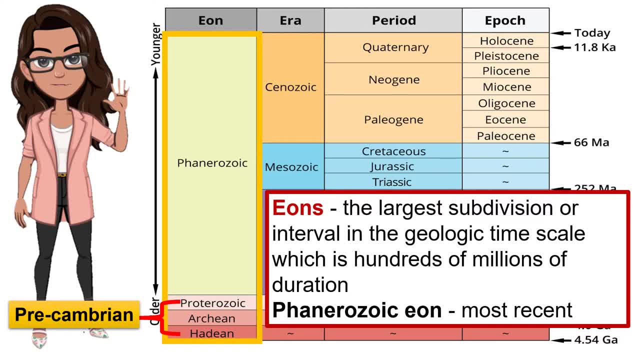 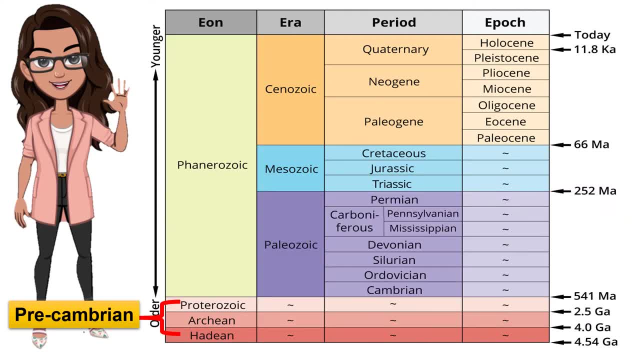 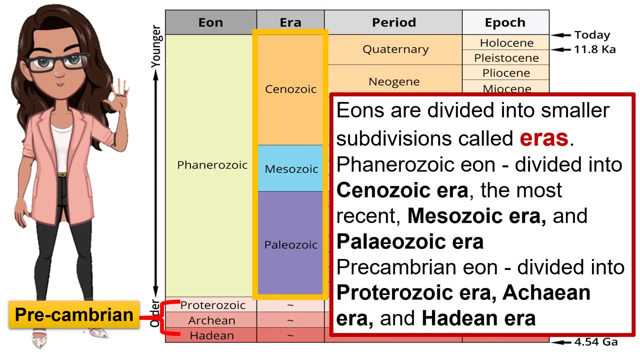 most recent geologic time scale. in the geologic time scale, which is hundreds of millions of duration, the panerozoic eon is the most recent, which is about 500 million years ago. then the Precambrian eon eons are divided into smaller subdivisions, called you Elas. the fatнопic eon is divided in 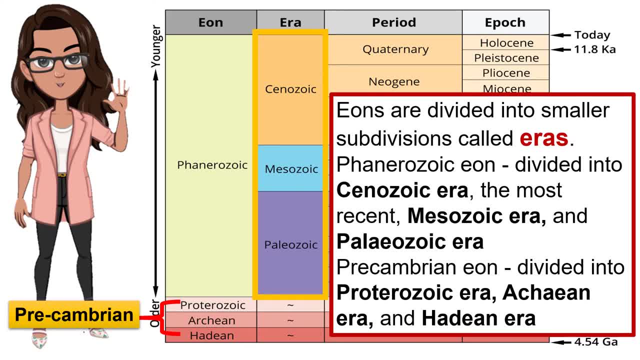 two center Zoe kira, the most recent about 65 million years ago. Mesozoic era occurs between 6- 250 million years ago, while paleozoic era is about 299 to 542 million years ago. in precumbrian eon it is divided into proterozoic era, which is about 2 500 million years ago. 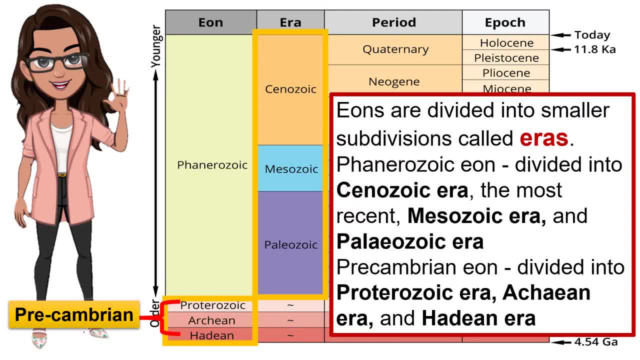 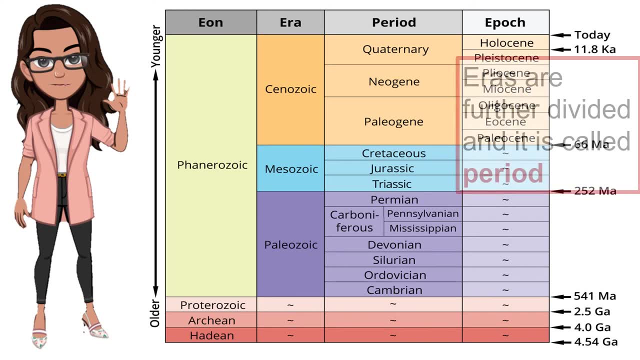 the archaean era 3 800 million years ago and the hadian era, which is 4 600 million years ago. next is periods. eras are further divided and it is called period in the geologic time scale. cyanozoic is divided into quaternary and tertiary periods. 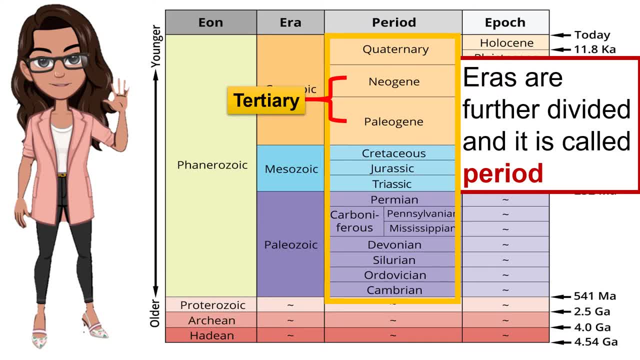 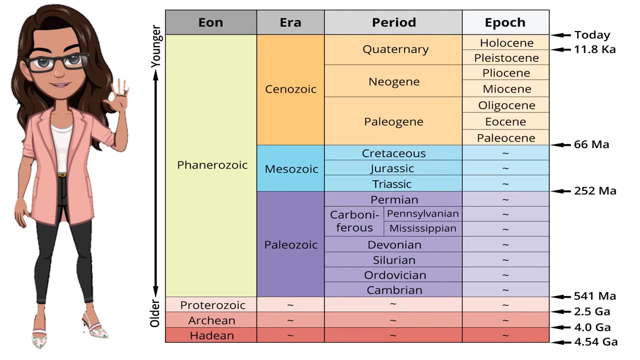 the mesozoic into cretaceous, jurassic and triassic periods, the paleozoic into permian, pennsylvanian, mississippian, devonian, silurian, ordovician and cambrian periods. next is epoch. periods are further divided and it's called epoch. only in cenozoic era is finally. 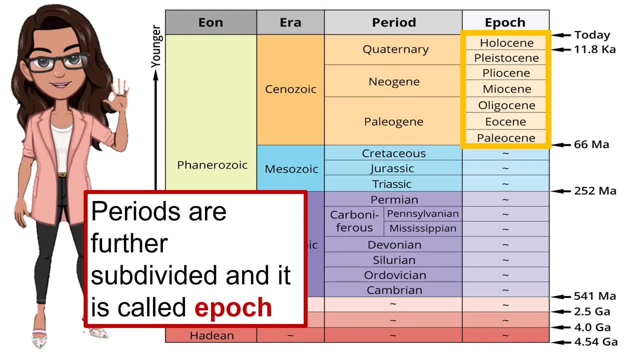 subdivided into epoch because rocks have been intensely deformed and are buried deeply and has been civilized in the plants of the earth. the period is called epoch because it is divided into epoch, because rocks have been intensely deformed and are buried deeply and has been civilized in the plants of the earth. 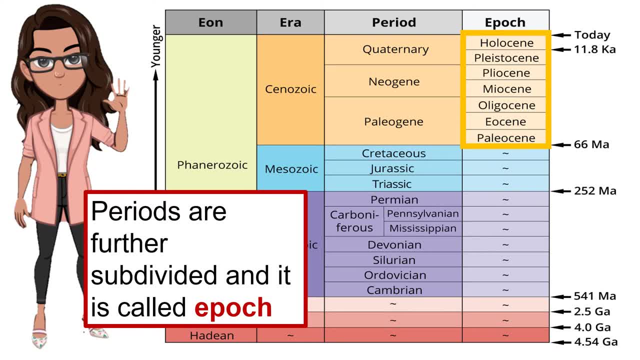 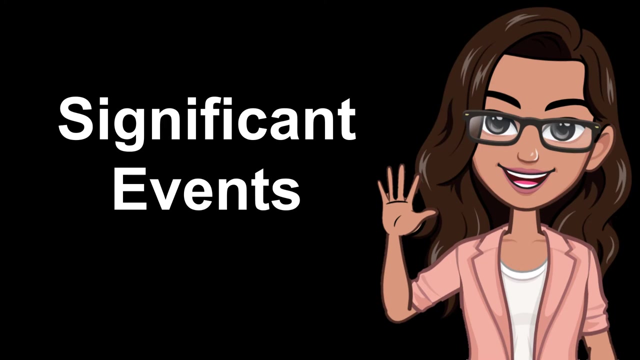 modified in a long-term earth process. the subdivisions of cenozoic era are for: quaternary period, Holocene and Pleistocene epochs, tertiary epochs, Pliocene, Miocene, Oligocene, Eocene, Pallicene epochs. now let's talk about the significant events that happened during the 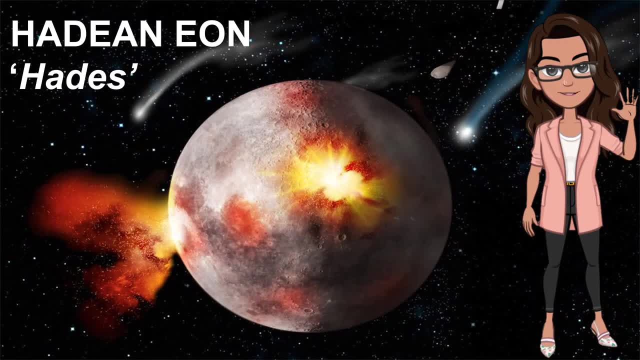 most recent part of the Earth's history. the enormous amount of events in the history of the earth happened during the Precumbrian, which is about 4.1 billion years ago. it was during Hadean, which came from the word Hades, meaning hell, was believed to be the origin of the earth. 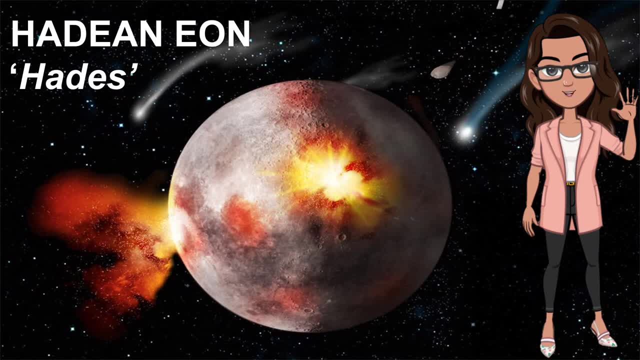 it was believed to be the most chaotic, due to the bombardment of meteorites in on earth, causing severe volcanic eruption. it was during this time when the ocean atmosphere and the core were formed, together with the stabilization of the crust. it is believed to be the beginning of the earth. 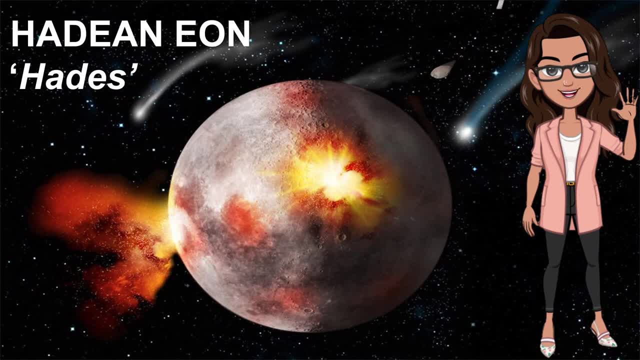 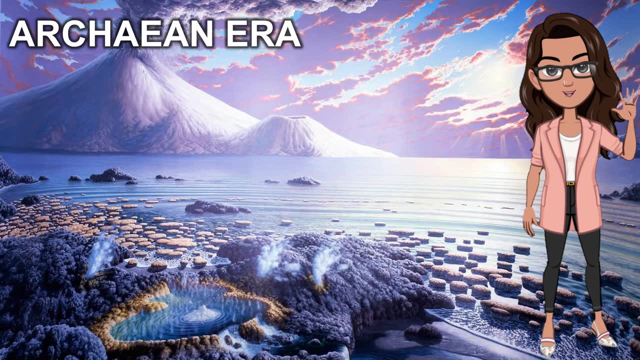 can you relate this with your lesson on the beginning of the solar system or the beginning of the universe? yes, yes, the Archean era was described as the time when the earth became warm. most of the earth was covered with water. methane gas occupied the atmosphere with little to no oxygen. the abundance of this 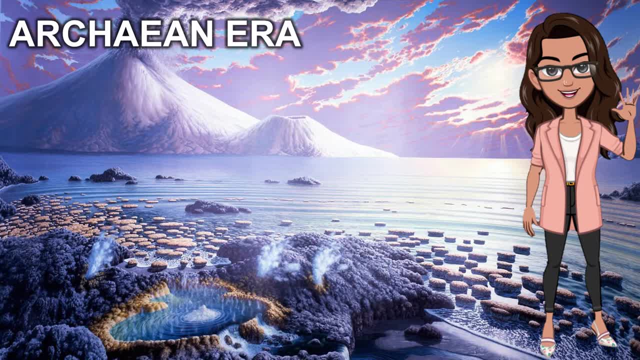 gas makes the atmosphere orange in color during this period. the formation of the continent was also believed to have started during this time, and great amount of iron and stromatolite on shorelines made the oceans green in color. maybe you are thinking about the seven continents that we have now. well, 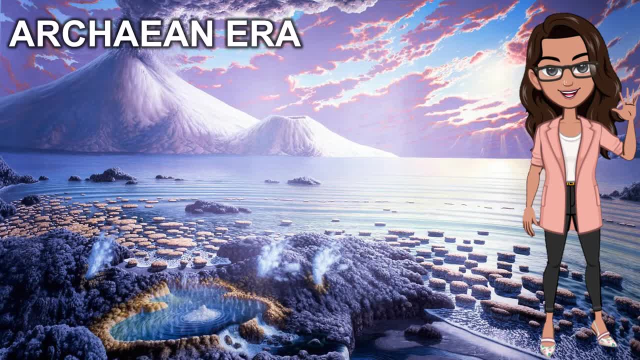 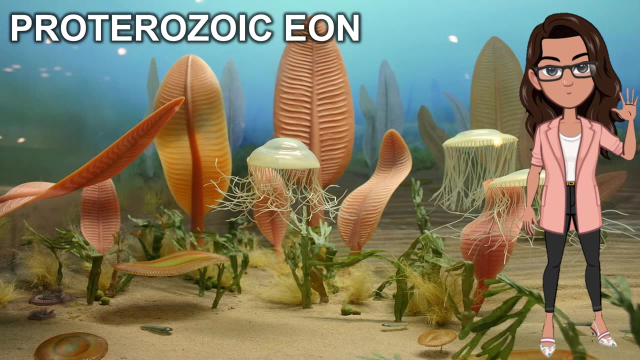 they are not the ones formed yet during this period. it is also believed that the origin of life, especially the prokaryotes, happened in this period in the produces week lasted almost half of the age of the earth. the atmosphere started to have oxygen making multicellular organisms called eukaryotes transformed удар multi-cellular animals also. 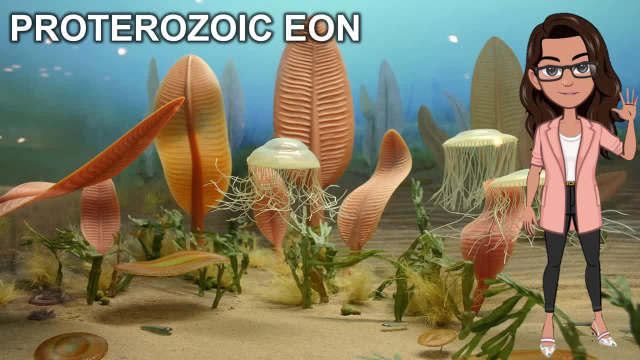 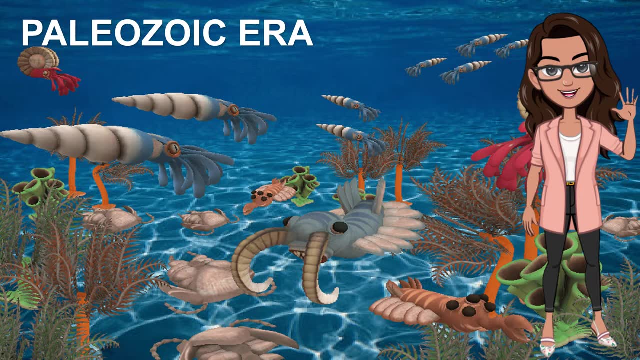 appeared at the continent started to drift away. TIP APOLOGY, lighting The skyline of the continent turned into a? d以及 UKRAINE Lauren's derechos imaginarium. segundo Stполож, powerful fenugreek of paleozoic era. life began to flourish in the sea. can you name some of the invertebrate that? 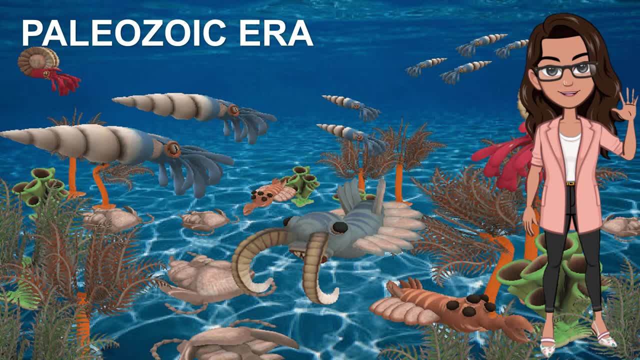 you know, they actually appeared during this era. that is why it is known to be the age of invertebrates. the fossils of marine invertebrates which lived near shallow waters were found to form in sedimentary layers. can you imagine a two-feet size cockroaches flying or creeping? 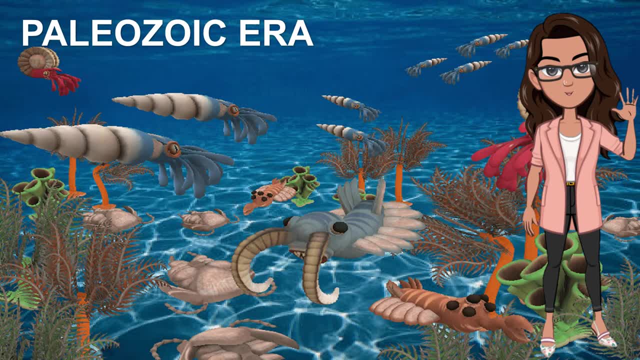 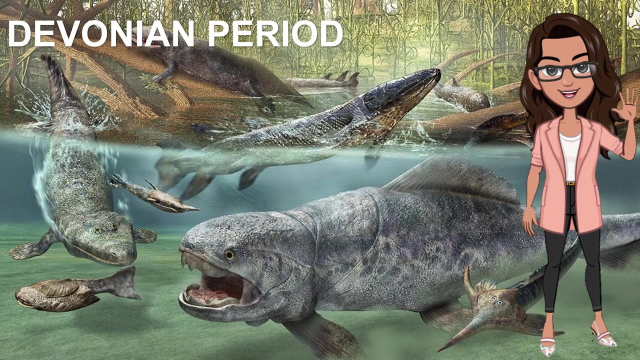 around now. actually, these are trilobites. trilobites appeared during this era. trilobites fossils were spotted to have been preserved in rocks during this period. in the midst of this era, animals that lived in water had developed shells at the time of Devonian period, which is known as. 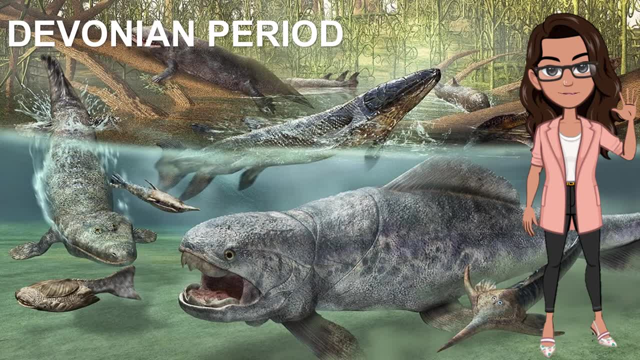 the age of fishes, plants and the first insect is believed to have evolved. animals started to breathe air as they came out of the sea and transferred to land, like the amphibians that you know now. land plants like the marsh plants and giant ferns began also to developed. in the late part of paleozoic era, reptiles started to 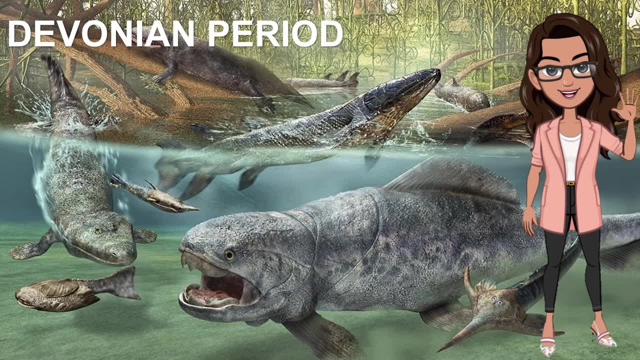 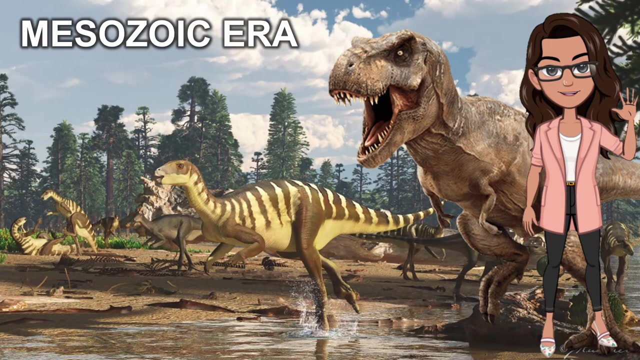 appear, which must like their amphibian ancestors, only that they were able to lay eggs on land. the remains of this formed the large amount of coal deposits in many areas of the world. at the time of early Mesozoic era, or also known as the age of dinosaur, marked the breaking up of 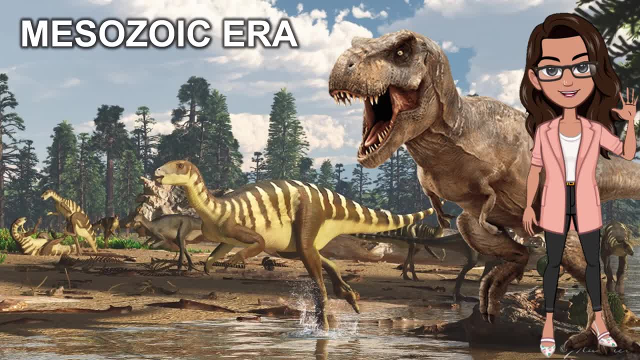 major land masses. the dinosaurs, the largest creatures that existed during this period and this believe to be the descendants of the early reptiles, survived throughout this era, said to know that these large creatures are already extinct and they are now just part of the history of the world. 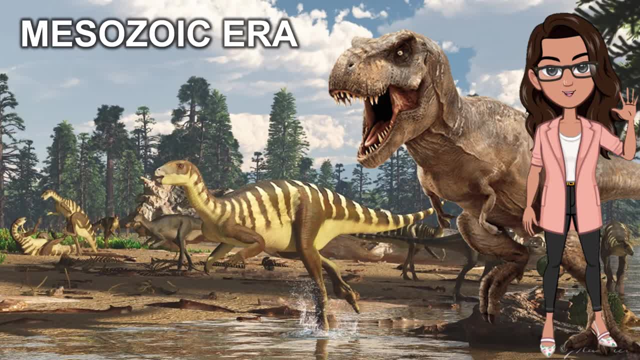 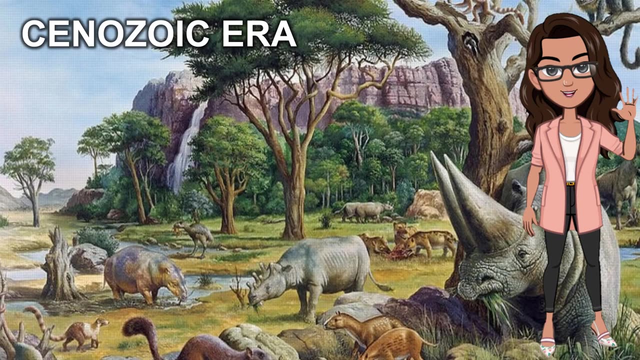 If you could have the chance to peep through this period, would you like to see the T-Rex, Or the Stegosaurus, Or Triceraptors? Hmm, sounds fun right? The Cenozoic Era, which is known as the Age of Mammals, new lifeforms started to appear. 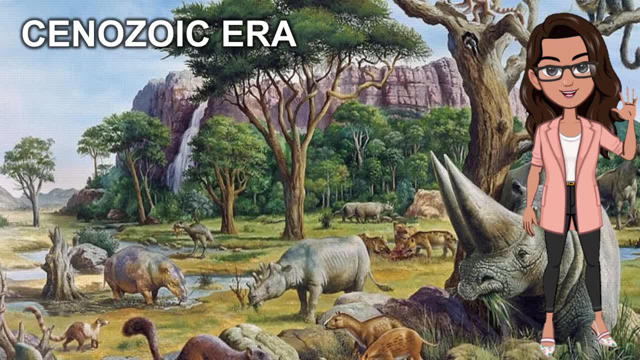 Volcanic eruption took place on a large scale, forming colossal flows of lava and basalt. Warm-blooded animals and other primordial mammals roamed the land. It was during this era, as observed in the stone tools used, that humans left marks on land. 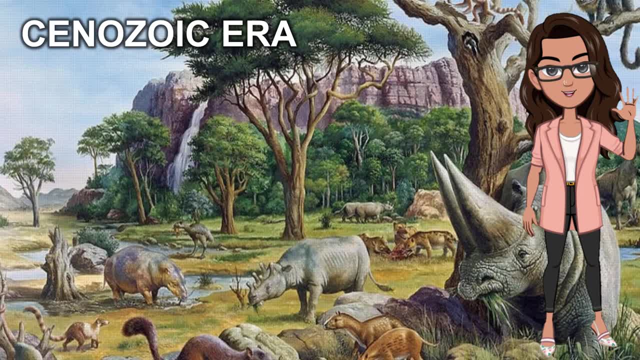 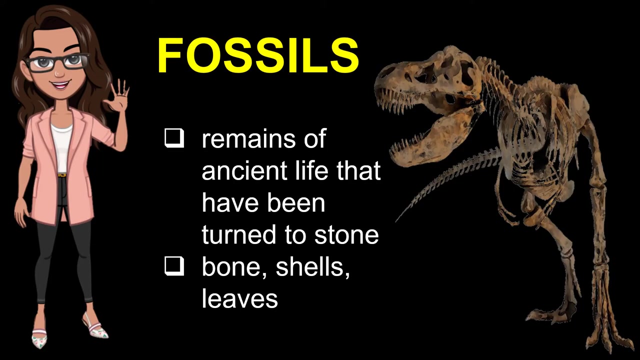 And so we are in this period. That's why we are here. Can you imagine how God prepared everything before the human being came? Wow, it is well-planned and systematically created. This time, let's talk about fossils. Fossils, as mentioned, are remains of ancient life that have been turned to stone. 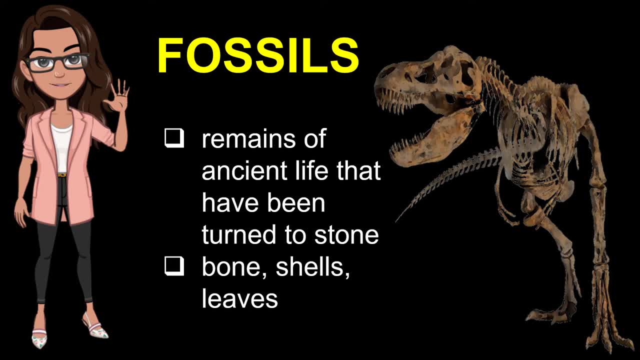 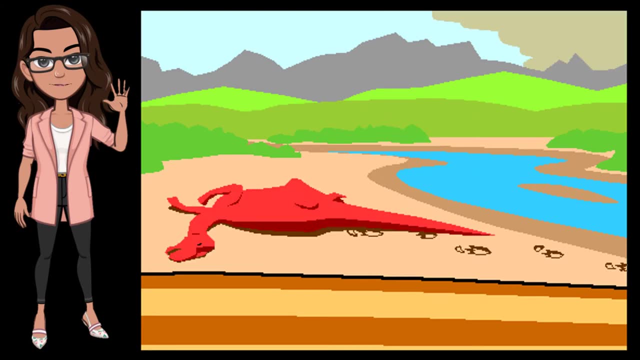 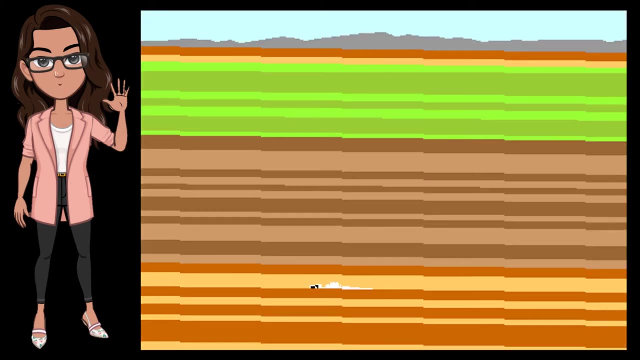 It can be actual parts of plants and animals, For example bones, shells and leaves. Most fossils are found in sedimentary rocks. These rocks form on the surface of the Earth. They record the processes that have happened on the surface, including life. 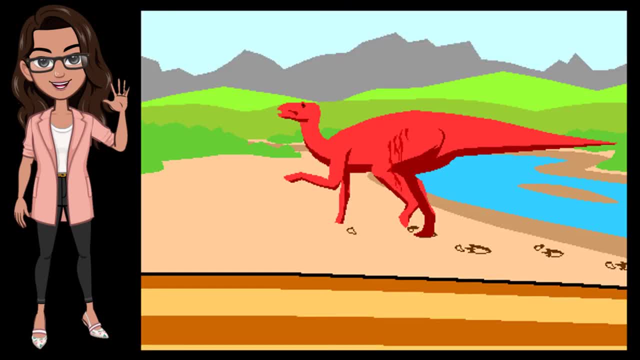 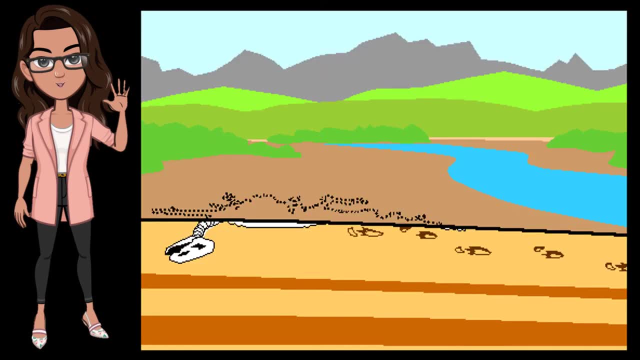 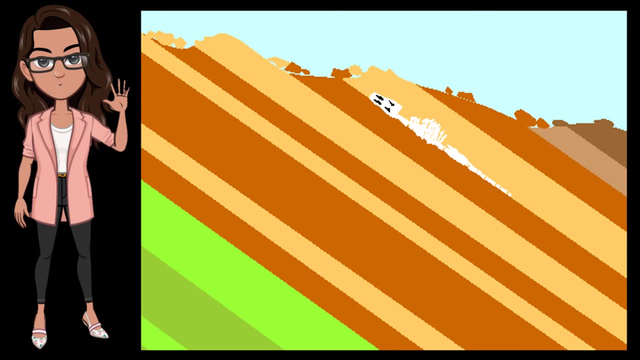 Scientists are able to arrange fossils according to their own knowledge. This is called the fossil record. By studying the fossil record, scientists have found that the Earth and its life forms have gone through many changes in the past. Fossils have taught us how and when rock layers have formed. 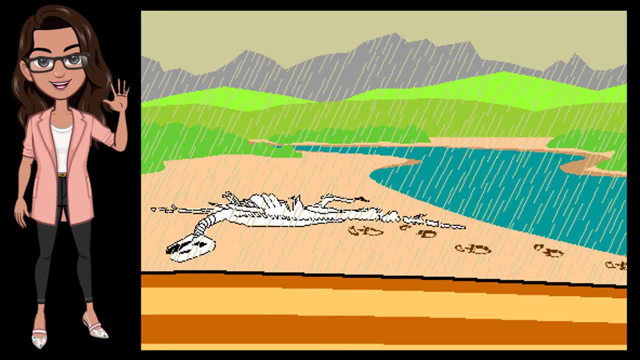 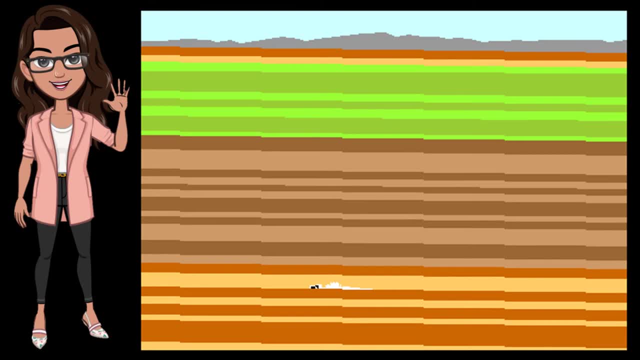 They also help scientists learn about life forms that have come and gone. Fossils have been taught about life forms that have come and gone. They also teach us a lot about the planets and their solids. Students have been taught about the climate of the Earth long ago. 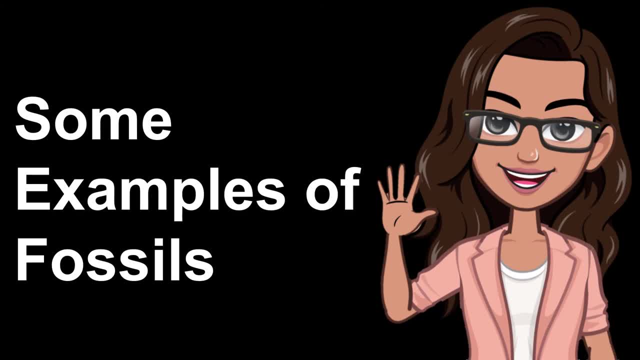 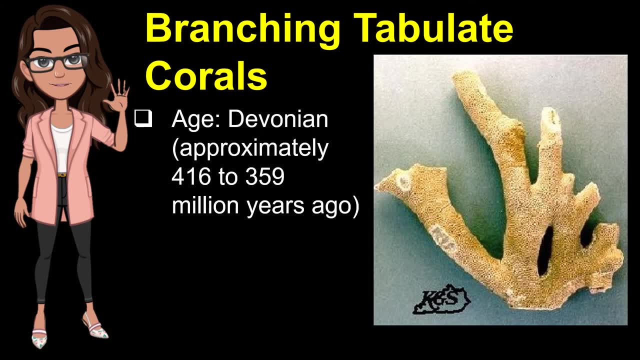 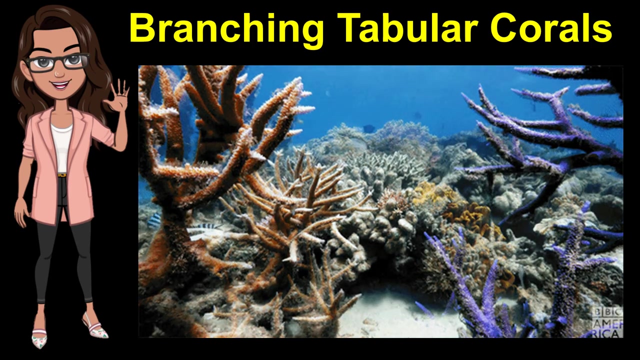 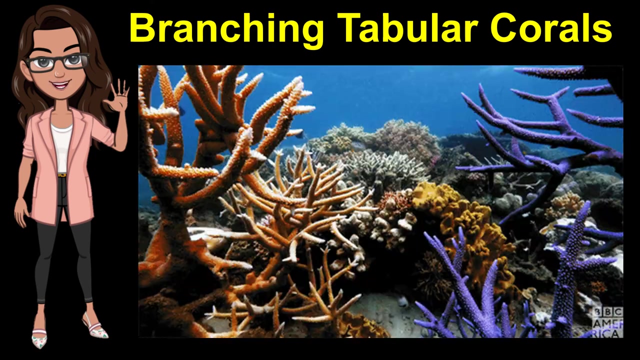 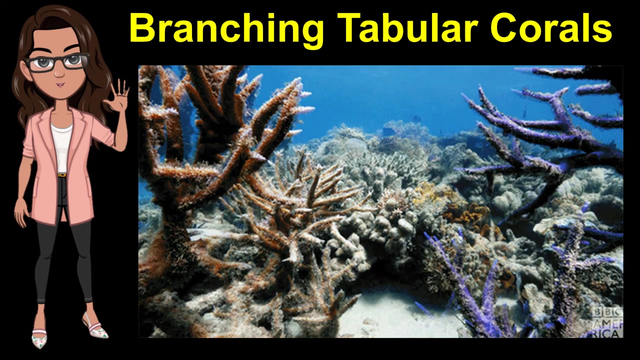 Here are some examples of fossils: Branching tabulate coral, Devonian Approximately 416 to 359 million years ago, Underclass anthozoa anthozoa. the modern relatives corals still exist today. this is a branching tabulate coral. a branching tabulate coral is a marine animal. corals are multicellular organisms that often 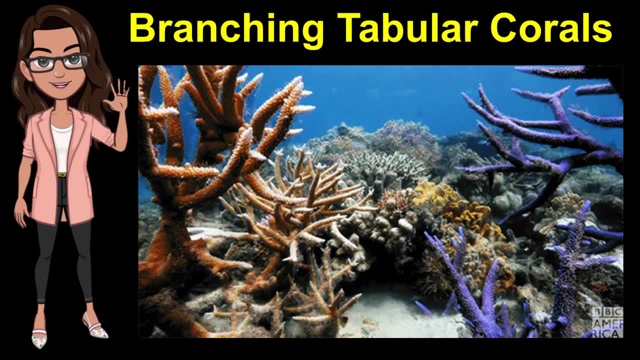 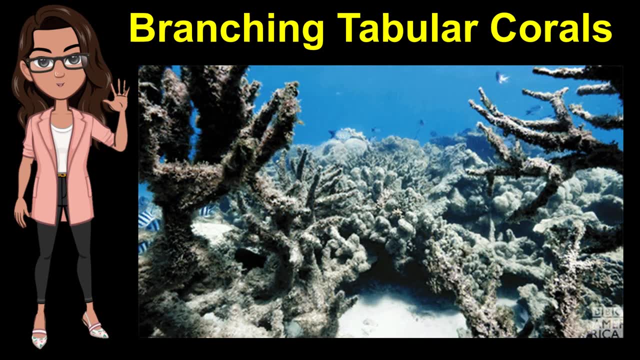 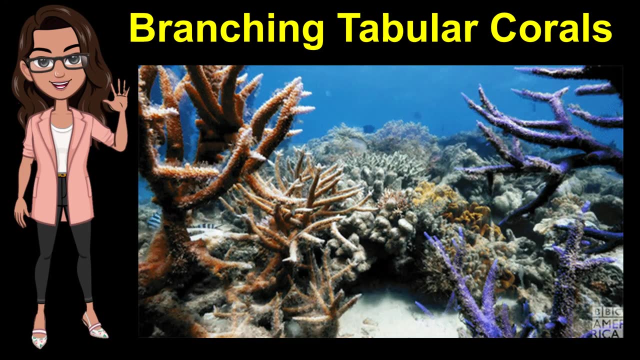 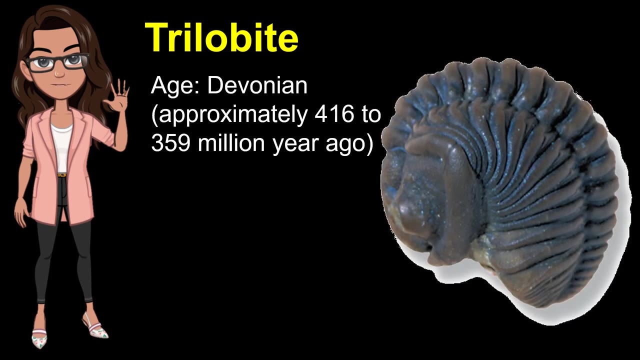 live in colonies. the individual animal is called a polyp. there are many different species of coral with different forms, shapes and sizes. next is a trilobite, age devonian, approximately 416 to 359 million years ago. phylum arthropod, the modern relatives, crabs, spiders and insects. trilobites were marine arthropods. the first trilobites show up in the fossil record dating back to about 525 million years ago. There were many different types of trilobites, ranging in size from 1 millimeter to 72 millimeters or 28 inches long. Trilobite species went extinct by 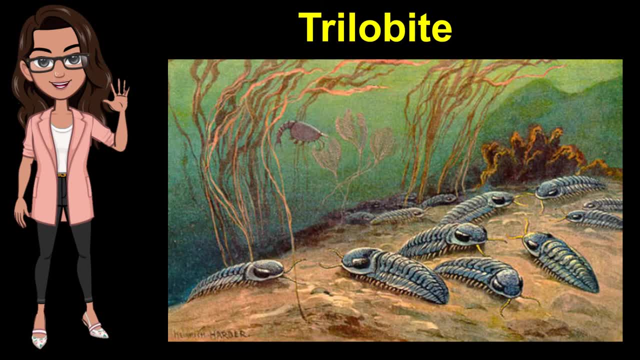 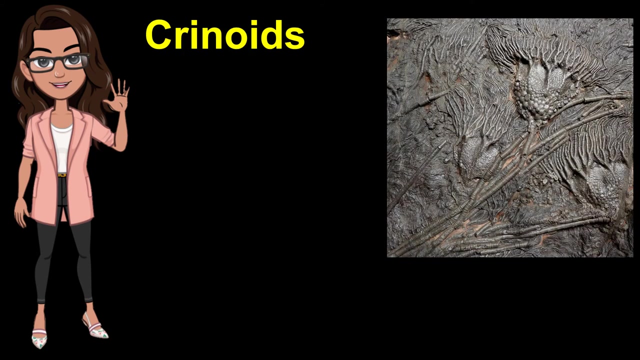 250 million years ago. Trilobite fossils are formed from the exoskeletons. These were made of chitin. like some insects and other organisms like lobsters, They split apart and shed their shell as they grow, just like lobsters do. Next is crinoids: Age devonian, approximately 416 to. 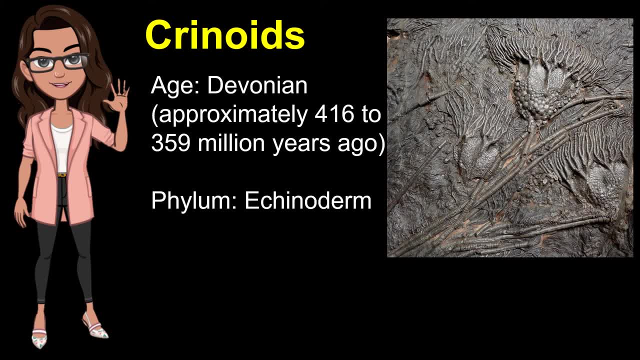 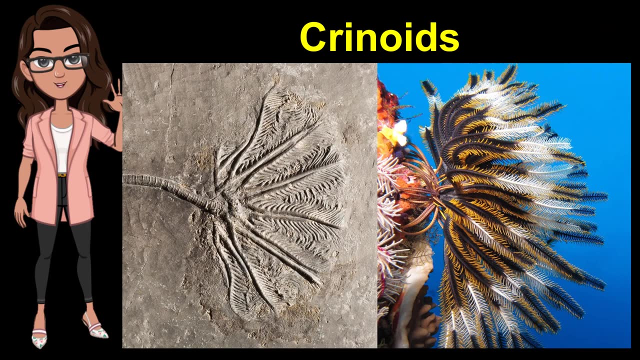 359 million years ago under phylum Echinodermata. Modern relatives are starfish, sea urchins and sea cucumbers. Crinoids were marine animals. Its name means lily. It is in the same phylum or Echinoderm as starfish. 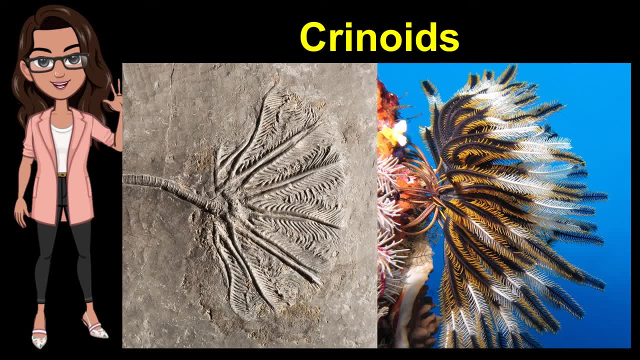 and sea urchins. Crinoids ate by filtering food out of the water with its arms. Its mouth and anus were next to each other. Crinoids ate by filtering food out of the water with its arms. Its mouth and anus were next to each other. 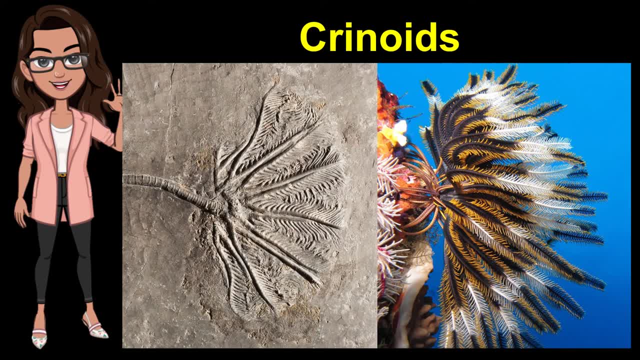 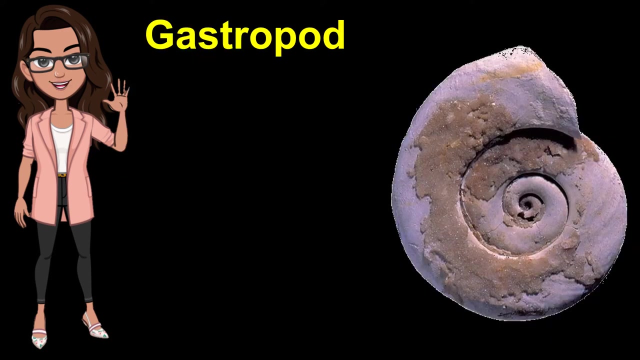 In the calyx. it rooted in place with the holdfast, and when crinoids die, their stems quickly break apart In the most common fossils of crinoids are the stem, which is sometimes broken into little cheerio-like pieces. Next is the gastropod Age Cretaceous, approximately 416 to 359 million years ago under phylum Echinodermata. Modern relatives are: age Cretaceous approximately 416 to 359 million years ago. under phylum Echinodermata, Modern relatives are age Cretaceous approximately 416 to 359 million years ago. under phylum Echinodermata, Modern relatives are: 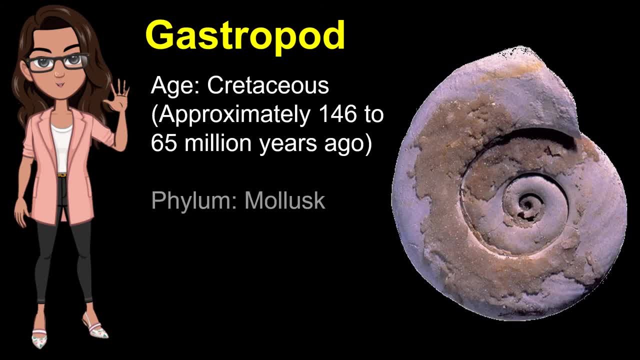 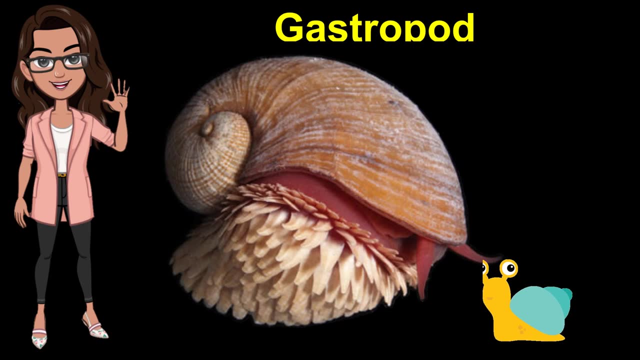 the Adamzwischenidae Around 5,500-6,000 năm ago. there were many different species of gastropods. All had coiled shells, But some were tightly-coiled, while some were loosely-coiled, which was long and expensive. 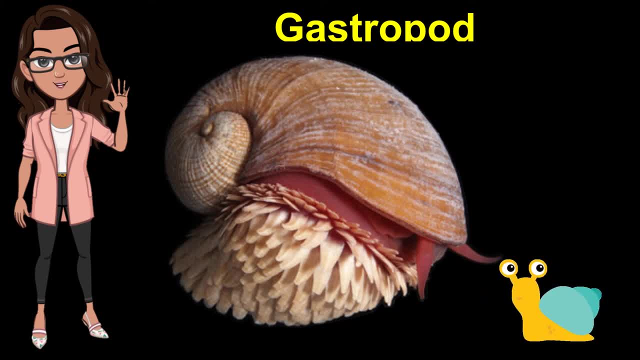 While some were needles, channels of passage were involved in their strength, Even from crinoids to the расск stateァ. Gog and acht are wrapped with a inoculation band If we say that a sociais have been discovered, which means the intermix of animal species, the difference of language, nature and 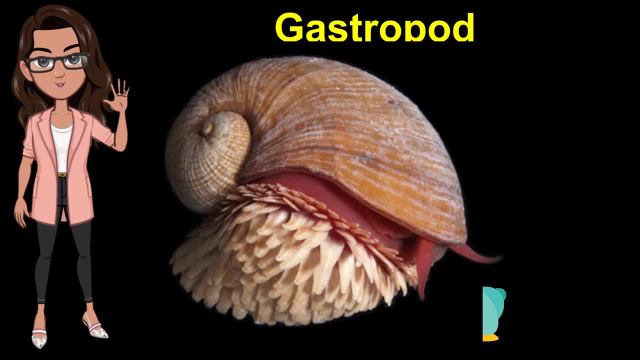 litigants of the food sector emerged after the extinction By 1844, betting on this pareil for beer. It was again conducted in the. They had many different shapes and surface texture. The animals lived inside their shells, taking up the whole inside of the long shell. 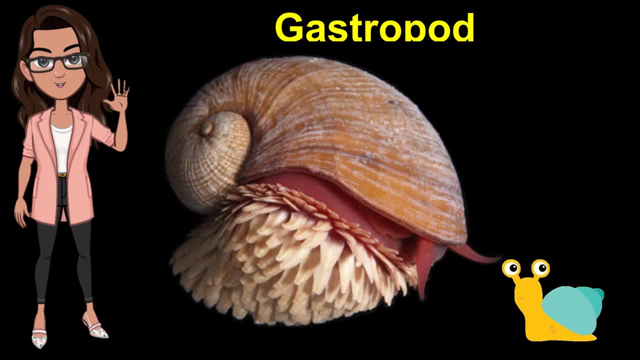 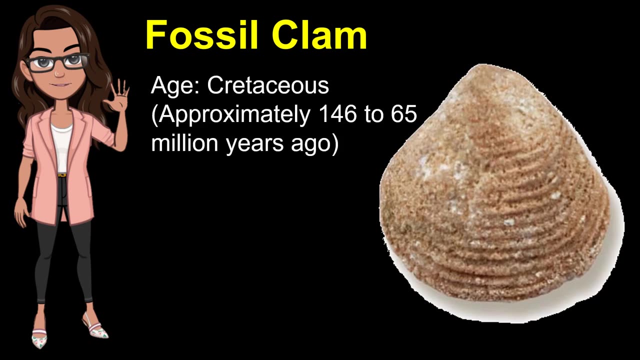 They could retract into their shells, covering the opening with their foot. This is the fossil clam. age Cretaceous: approximately 146 to 65 million years ago. class bivalve Modern relatives are oysters, scallops and mussels. 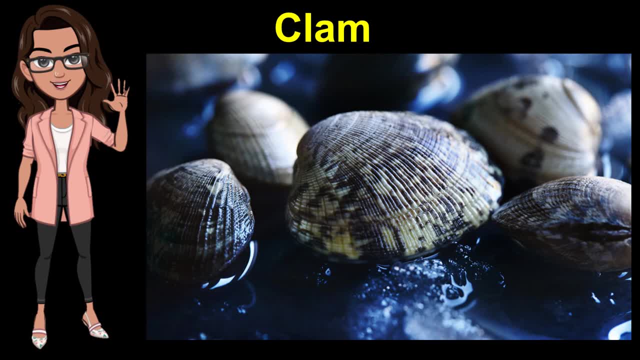 Fossil clams are marine animals. Clams are bivalves with two asymmetrical shells. The shells are mirror images of each other. Fossil clams range in size from a few millimeters to up to 2 meters, or about 6 feet in diameter. 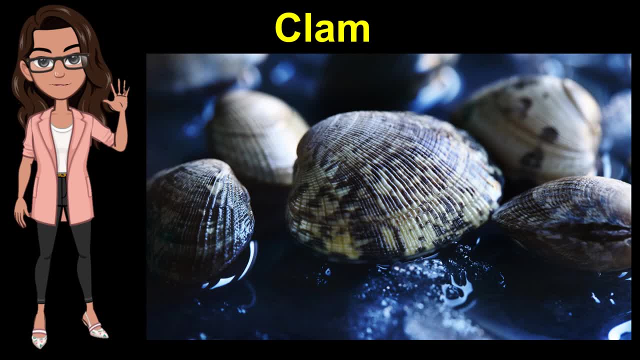 Clams lived inside their shells and had a muscular foot. they used to burrow and move around. They lived in colonies on the ocean floor. Some clams have smooth shells, while some are rough. Clams Clams, Clams, Clams.